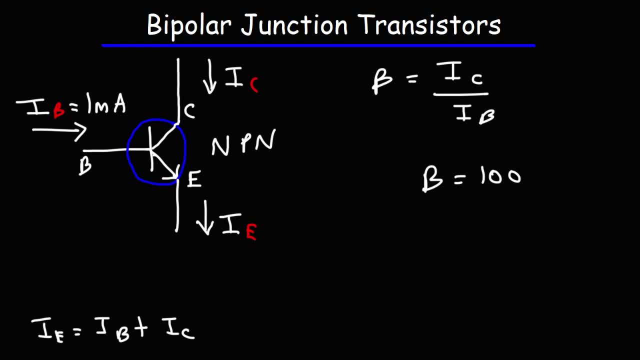 is actually in the opposite direction. So keep that in mind. Now, if the base current is 1 milliamp, what is the collector current? The collector current is going to be 100 times greater than the base current, So it's going to be 100 milliamps. So beta tells you the relationship. 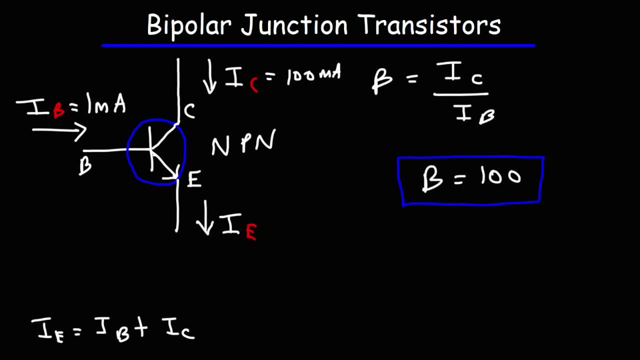 between the collector current and the base current. If beta was 200, the collector current will be 200 times greater than the base current, And so in this way, the transistor acts as a switch. You could use a very small current to activate a larger. 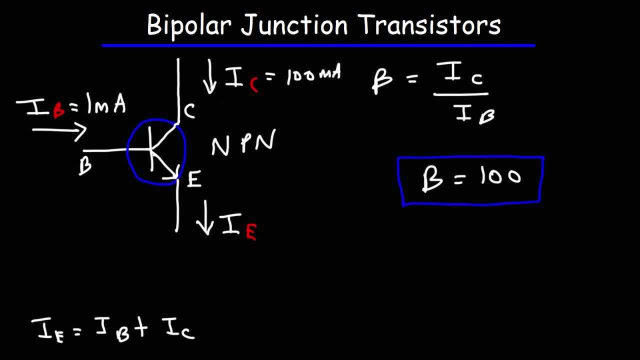 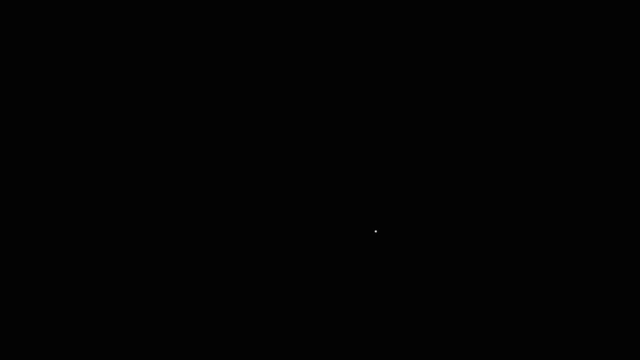 current in another circuit. Now the emitter current in this example is going to be the sum of the base current and the collector current, So that's going to be 101 milliamps. Now let's consider the PNP transistor. So notice that the arrow points towards the center of the transistor. 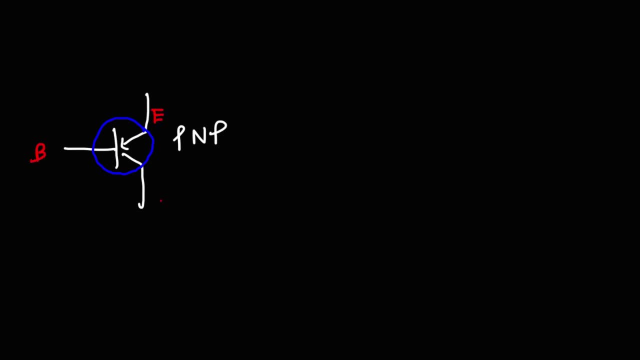 So this is the base, this is the emitter and this is the collector. So current is going to flow towards the emitter of the PNP transistor in the direction of this arrow. Now the base current flows out of the transistor In the NPN transistor. 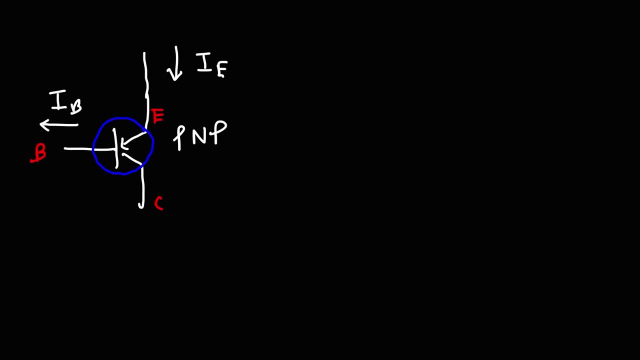 the base current flows into the transistor- That is conventional current- And the collector current flows away from the transistor. So beta is going to be 100 milliamps. So beta tells you that the collector current is going to flow towards the emitter of the transistor. 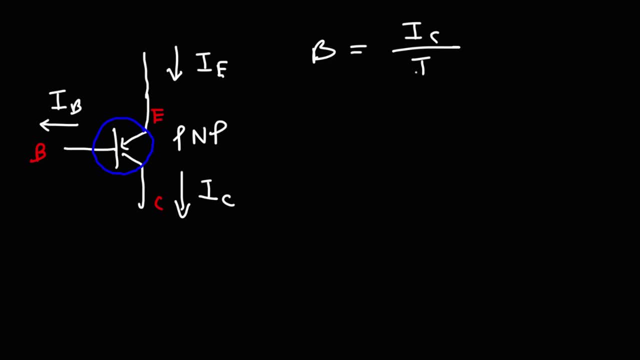 is still the ratio between the collector current and the base current, and the emitter current is still the sum of the base current and the collector current. so here's another example. let's say that beta is 200 and the base current- we're going to say it's 2 milliamps. go ahead and calculate the collector current and 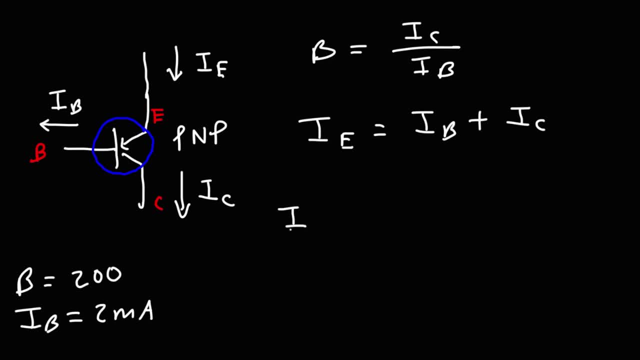 the emitter current in this example. so the collector current is going to be beta times the base current, so it's 200 times 2 milliamps, which is going to be 400 milliamps, and then the emitter current is going to be the sum of these. 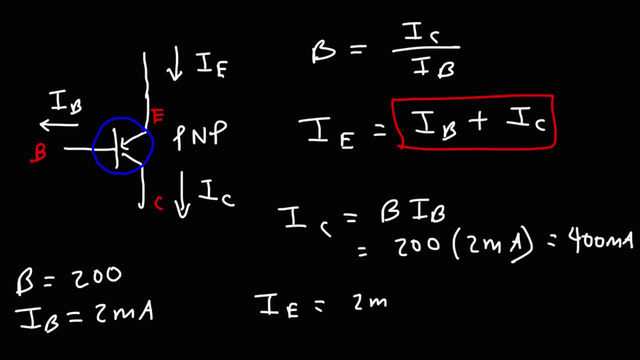 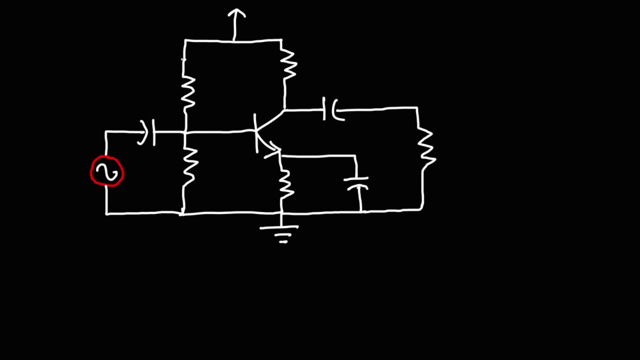 two currents, so that's going to be 2 milliamps plus 400, which gives us a sum total of 402 milliamps. so those are some basic calculations that you're going to encounter when dealing with NPN and PMP transistors. so what we have here is the common emitter configuration of a. 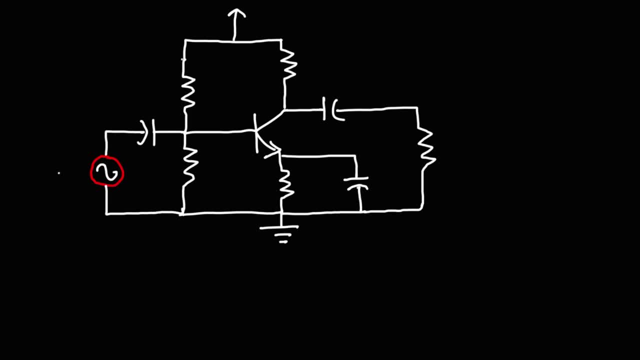 transistor amplifier. so this is the input signal and the output signal will be across the load resistor. the input signal is applied to the base of the transistor and the output is taken from the collector. now the emitter of the NPN transistor is common to both the input and the output circuits. 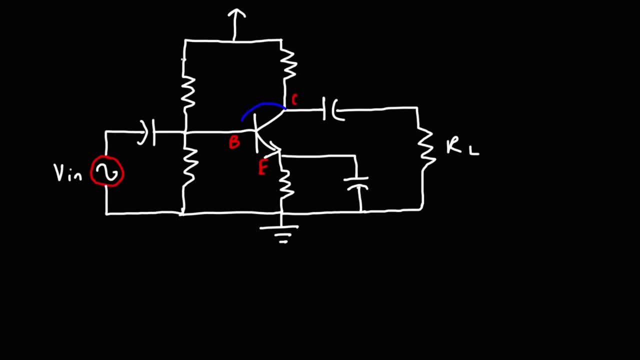 so that's why it's called the common emitter amplifier circuit. so this is the emitter resistance and this is RC, the collector resistance. this is R1 and R2. Those two resistors form a voltage divider circuit. CB is the bypass capacitor. It allows the AC signal to basically bypass. 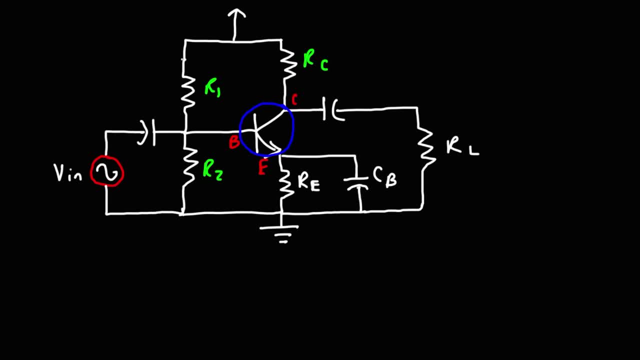 RE. This increases the gain of the amplifier. And then C2, that is the capacitor that blocks the DC signal but allows AC signal to pass to the output. And C1 does the same thing: It blocks the DC power from going into the input circuit while allowing the AC signal to pass through. 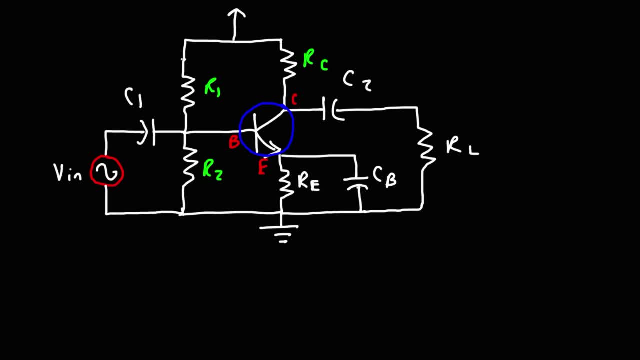 C1 to get to the transistor. So C1 and C2, they basically block the DC signal or the DC current that comes from the battery or the power source, But allowing the AC signal to pass through the circuit. Now let's say that the input voltage is 10 millivolts and the current we're going to say is: 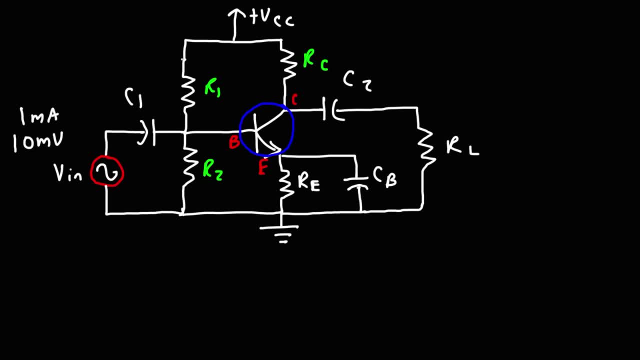 1 milliamp. Now let's say for a certain set of R1,, R2, RC and RE values. let's say that the output voltage, that is the output AC voltage across RL, we're going to say it's 400 millivolts And we're going to say the current is 15 milliamps. 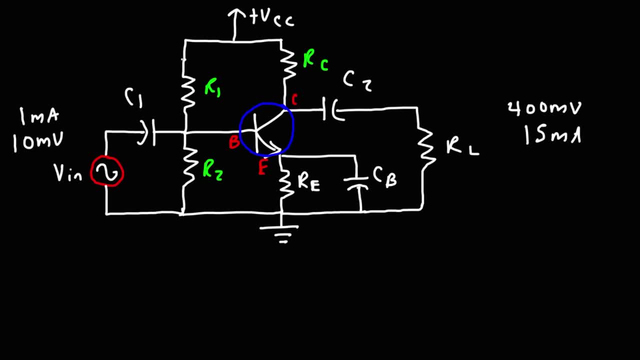 With this information, what is the voltage gain of the circuit And what is the current gain of the circuit? The voltage gain of the circuit, represented by AV. it is the ratio of the output voltage divided by the input voltage. So the output AC signal has a voltage of 400 millivolts. 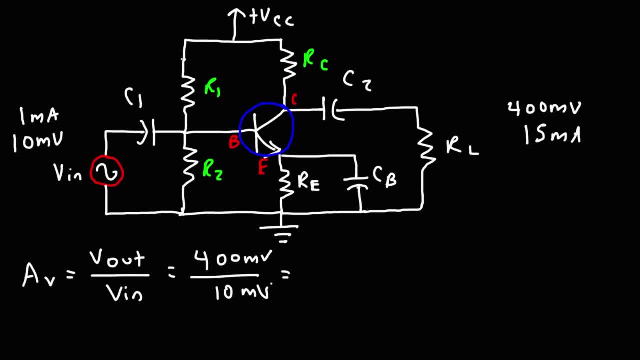 The input voltage is 10.. So for this example, based on these numbers, the voltage gain would be 40. Now the current gain is going to be the ratio between the output current and the input current of the AC signal. So the output current is 15 milliamps, The input current is 1 milliamp. 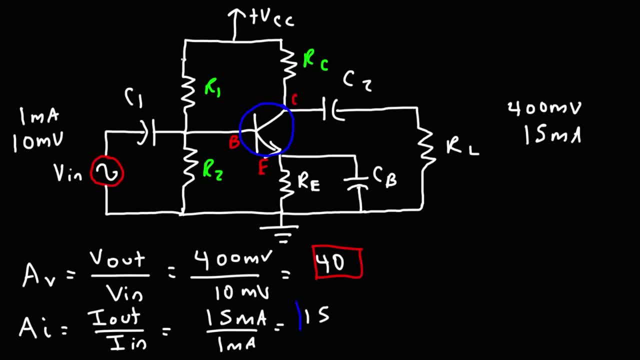 So then the current gain is 15.. Now the next thing we could calculate is the power gain. So to calculate the power, let's get this in voltage first. So we have 10 millivolts, which is 0.01 volts times 1 milliamp, or 0.001 amps. 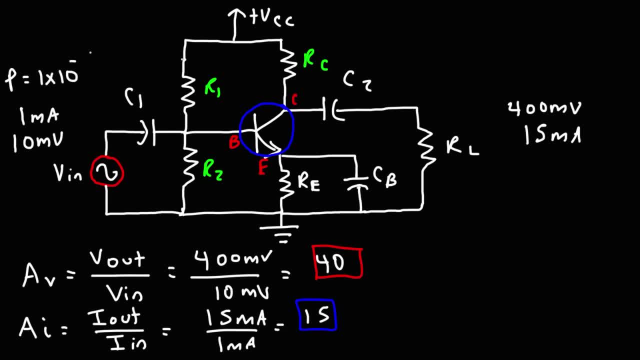 So the power at the input is 1 times 10 to the minus 5 watts. Let's convert this to milliwatts, Which let's convert that to milliwatts, So that's 0.01 milliwatts if we multiply that by a thousand. 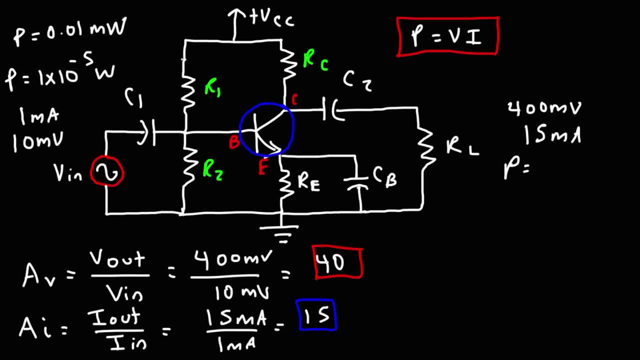 Keep in mind, power is a voltage times current. So now let's calculate the power at the output. So the power at the output is 6 times 10 to the minus 3 watts. If you multiply that by 1,000, that will give you 6 milliwatts. 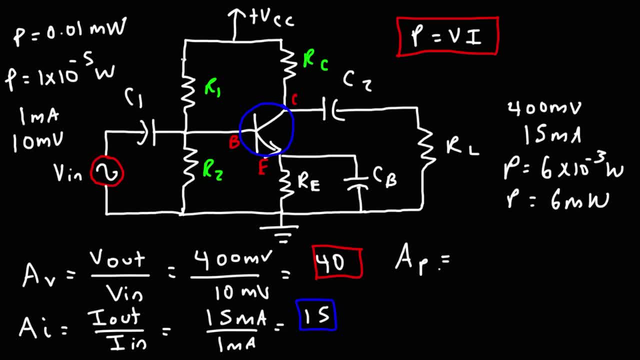 Now let's calculate the power gain. So that's going to be the output power divided by the input power. So we have an output power of 6 milliwatts and an input power of 0.01 milliwatts, And so this is equal to a power gain of 600. 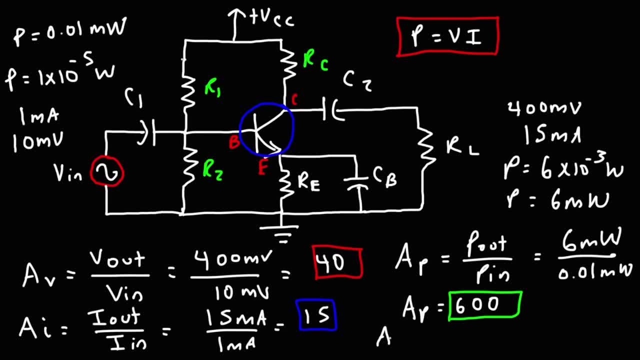 Another way in which you can calculate the power gain is by multiplying the voltage gain by the current gain. Okay, Because power is voltage times current. So 40 times 15 will give you 600 as well. So this helps us to see the characteristics of the common emitter amplifier. 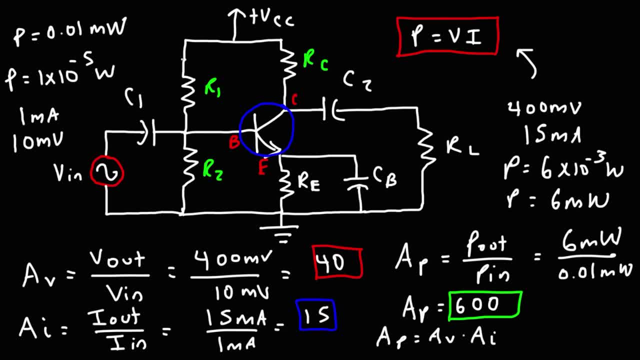 The common emitter amplifier has a mid-range current gain. It also has a mid-range voltage gain, but it has a high power gain, as you can see from this example. So that's one of the advantages of using The common emitter amplifier over the common base amplifier or the common collector amplifier is because it has a high power gain. 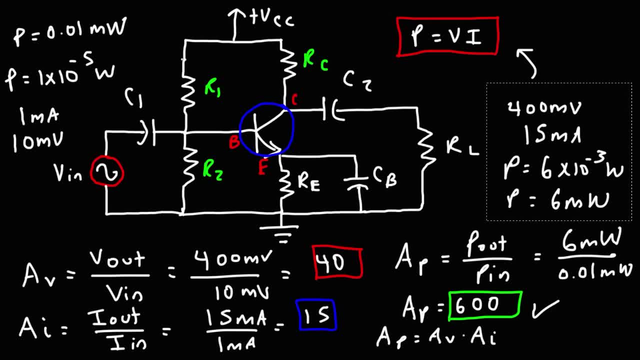 Now there's one more feature of the common emitter amplifier that I do want to discuss in this video, And that is the inverting characteristics of this amplifier. So at the input we may get a signal that looks like this: A nice sine wave. 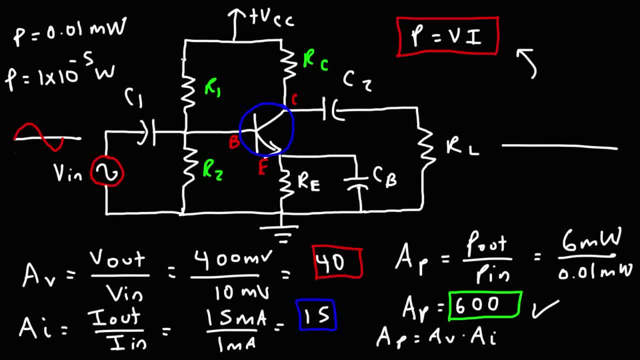 And at the output We're also going to get a sine wave, but it's going to be inverted. Basically it's shifted 180 degrees, but the amplitude is larger because it's been amplified. So that's. another characteristic of the common emitter amplifier is that it shifts the input signal by 180 degrees. 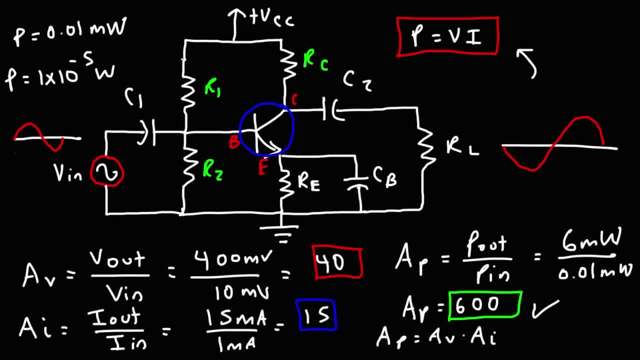 So when dealing with a sine wave, it looks like the signal has been inverted. So that's basically it for this video. Hopefully gave you a good introduction into the common emitter amplifier And how basic BJT amplifiers or BJT transistors work. 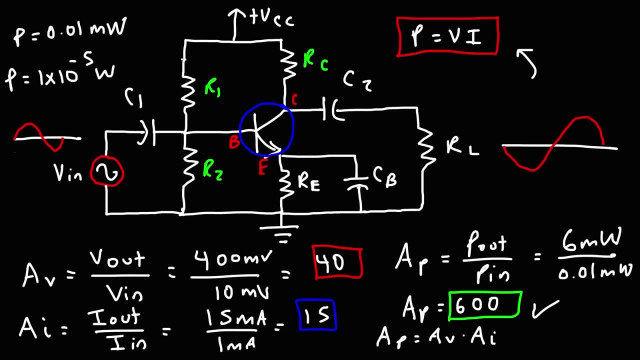 So now you know the difference between an MPN transistor and a PMP transistor and how the current flow into and out of these devices.